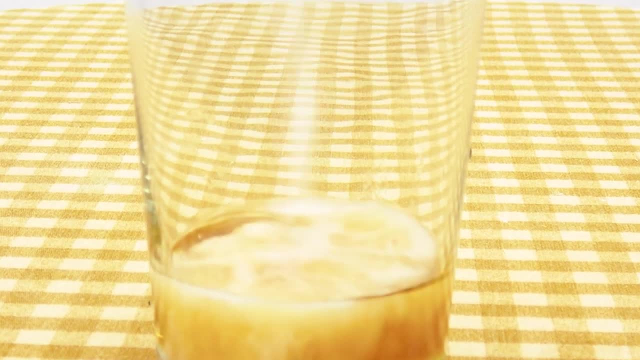 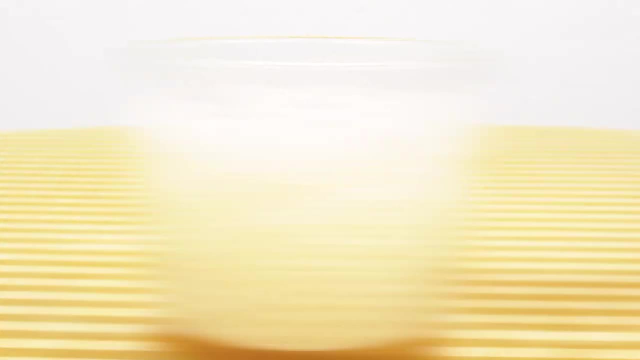 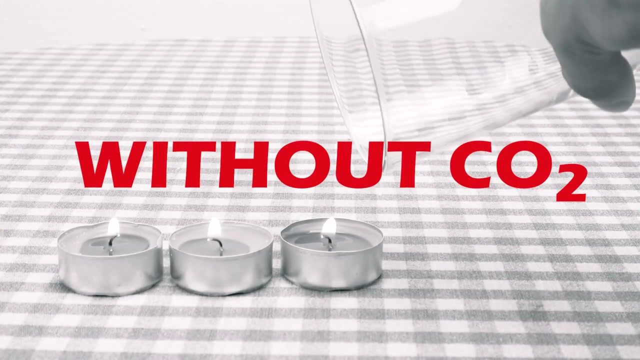 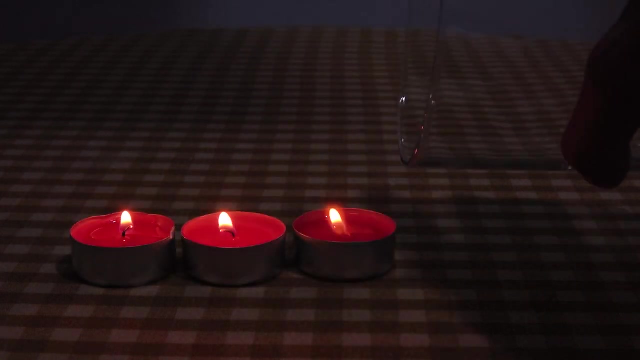 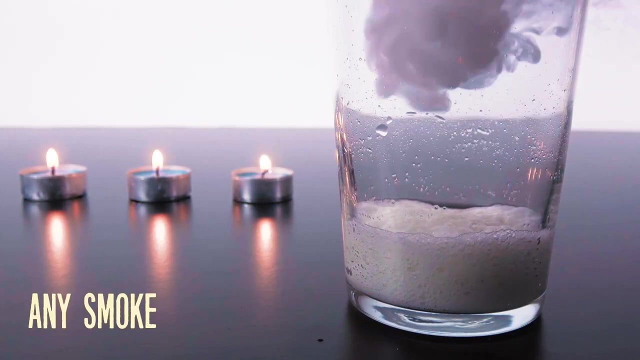 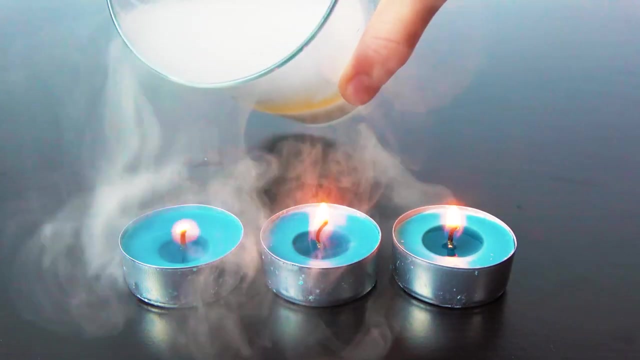 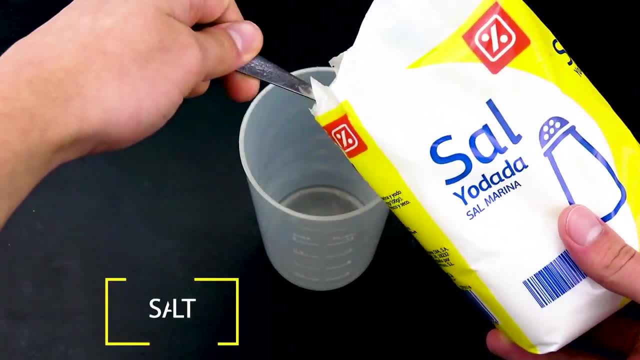 I take shots. I take loss. I make shots, I miss lots. I tell you, get big box to get yachts, just swing lots and pop off a big shot. I ain't done chasing, got big dreams, bigger things, impatient. 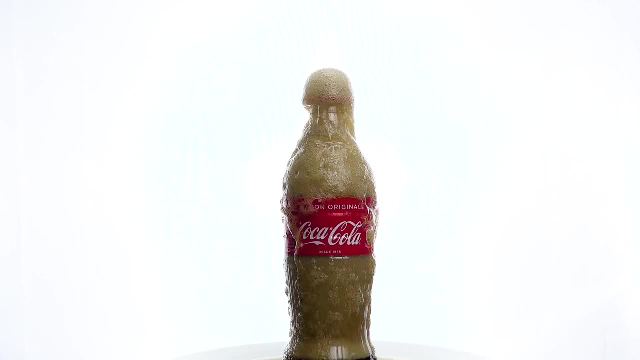 Who's at the top think they need replacement? Who's at the top think I'm gonna erase them? Face it. I don't give up quick. I don't give a shit. I won't give up this, cause I know that I want it. 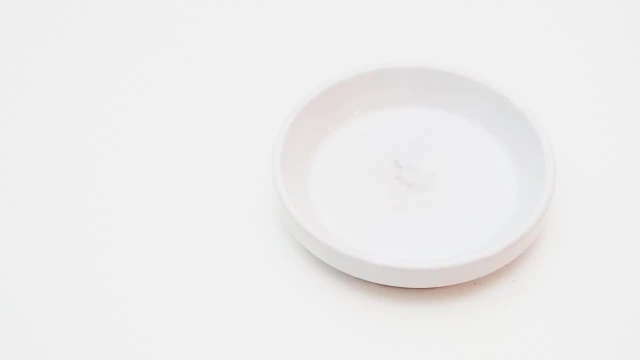 Know that I'm on it. I'll make it. I promise I won't give up this cause. I know that I want it. You don't wanna fuck with me. I slow burn like a disease. Just tell me that I can And I'll show you things that you couldn't be. 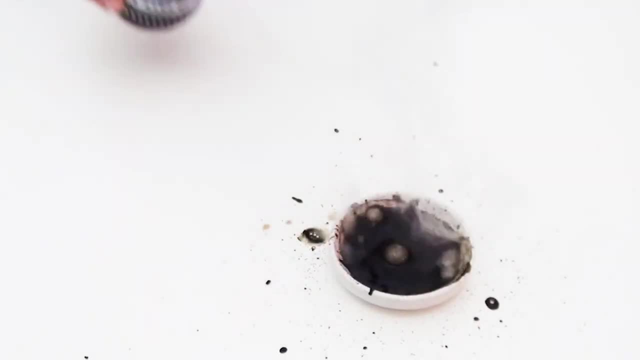 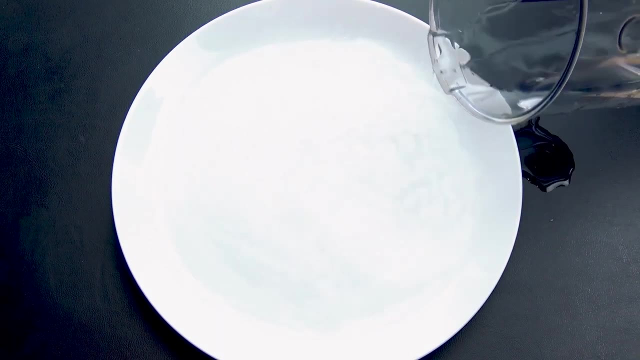 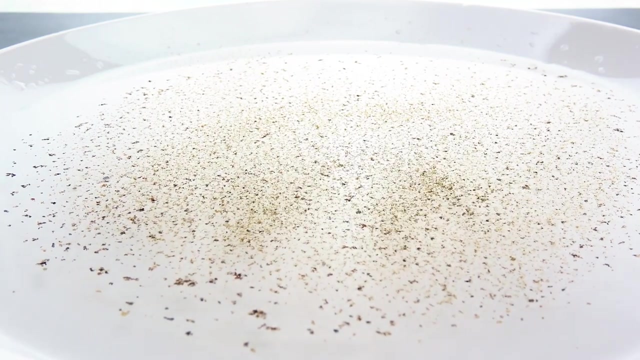 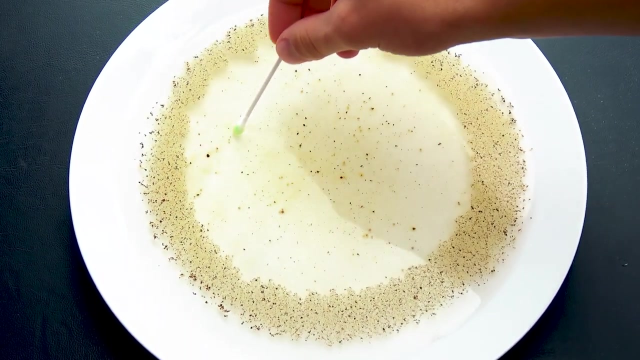 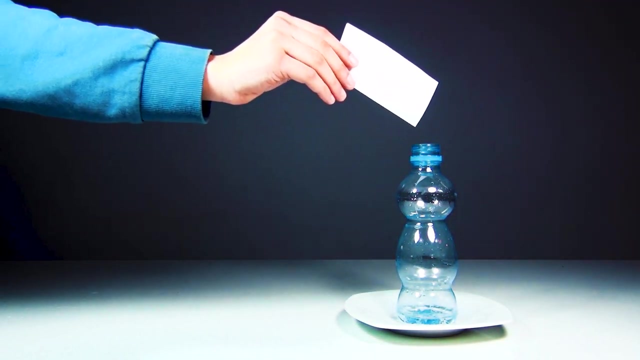 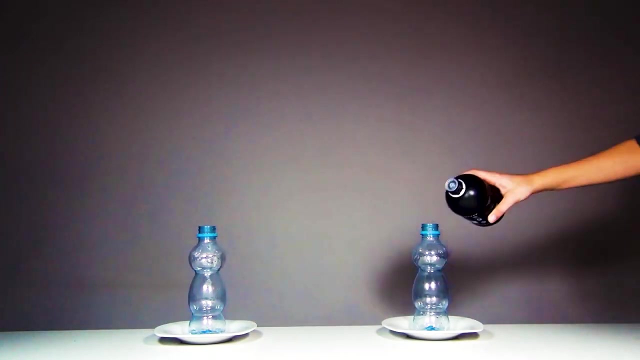 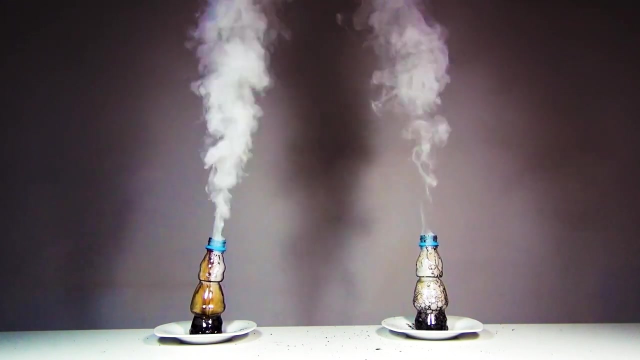 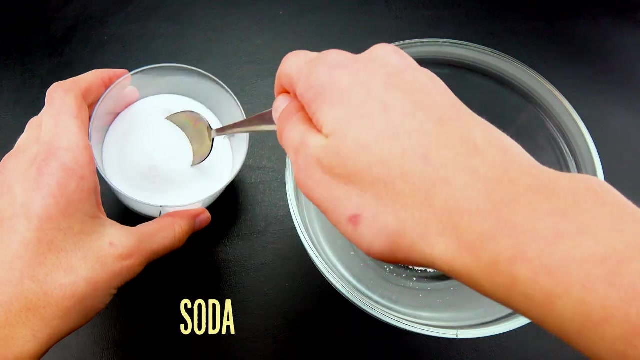 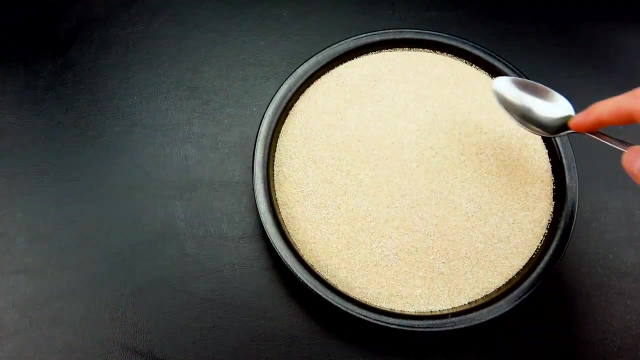 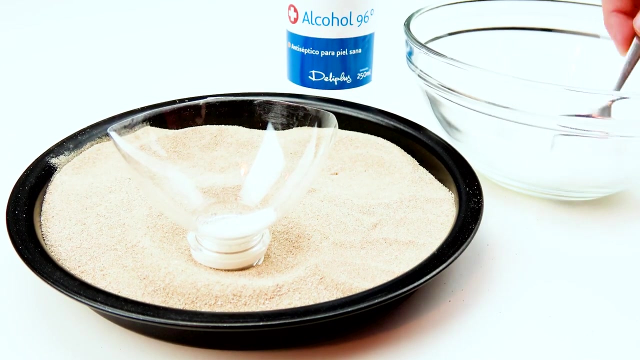 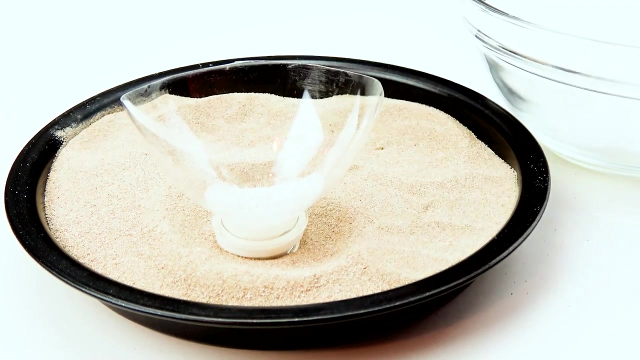 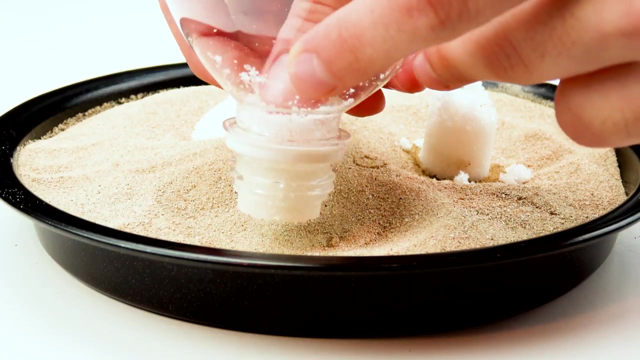 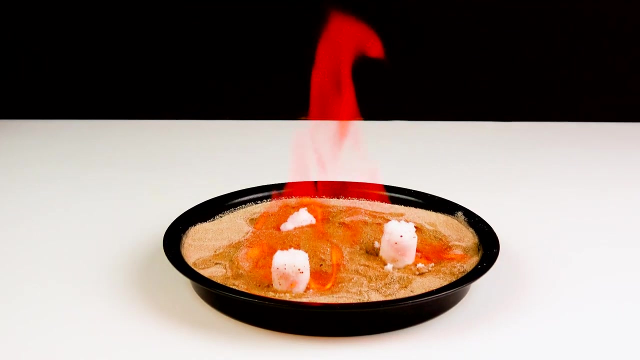 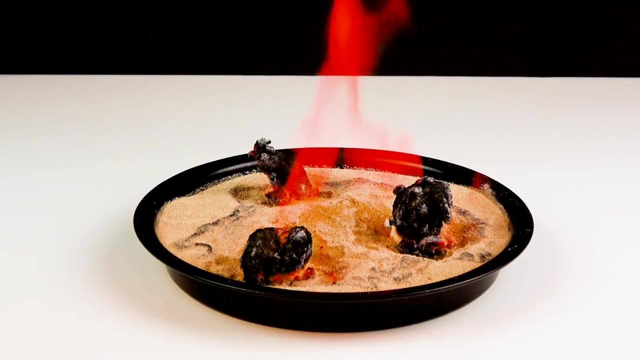 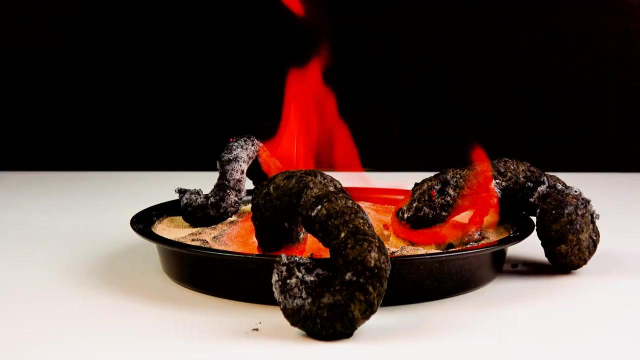 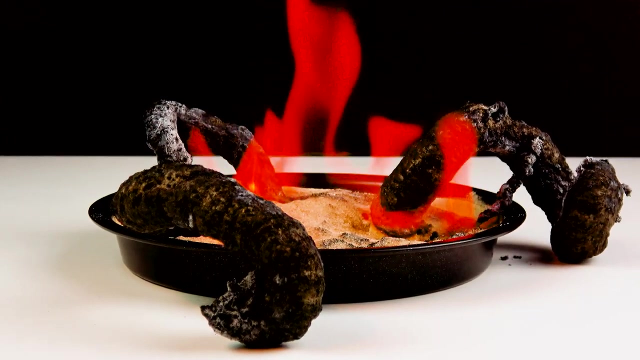 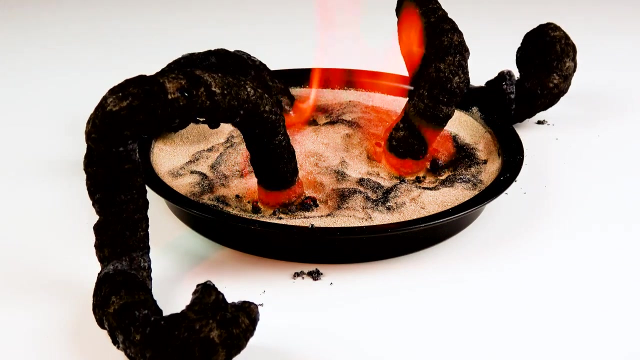 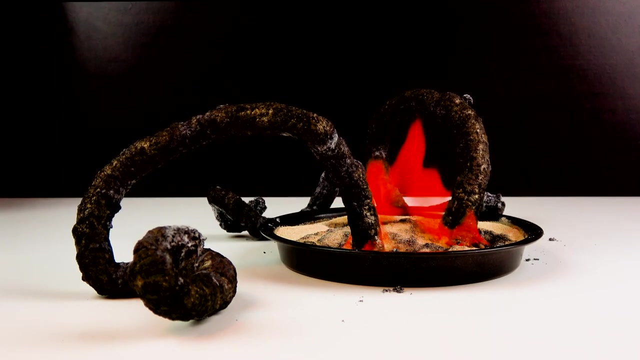 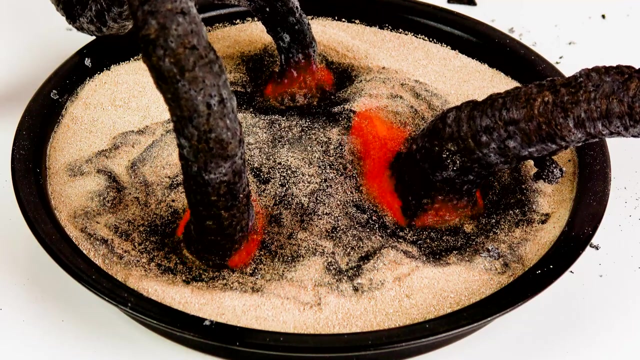 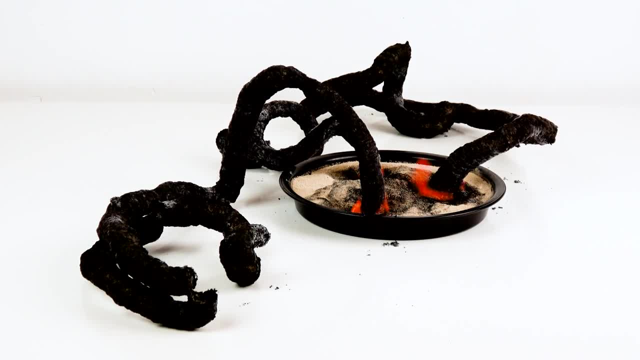 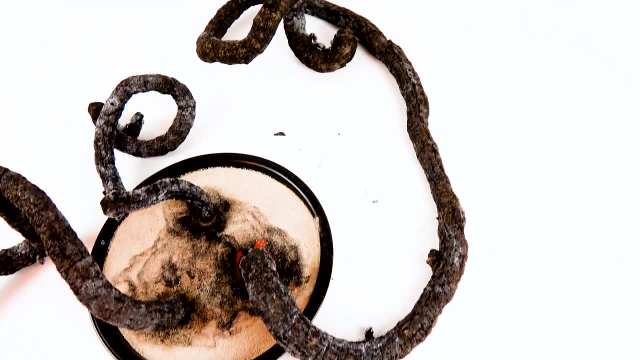 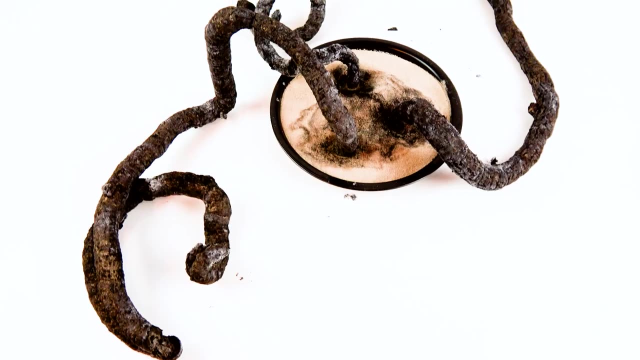 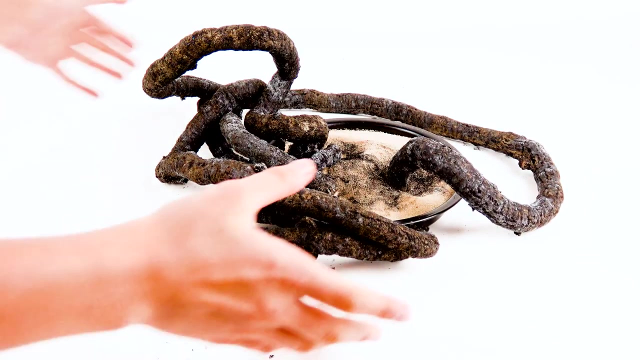 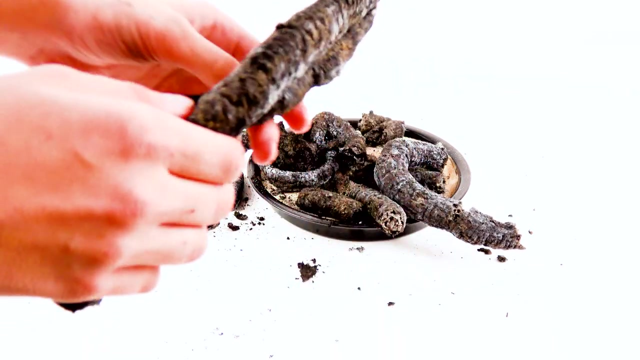 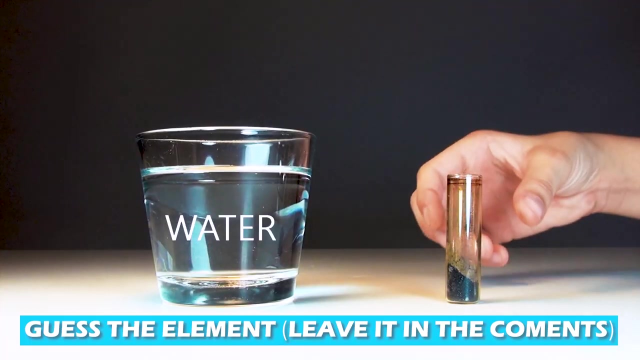 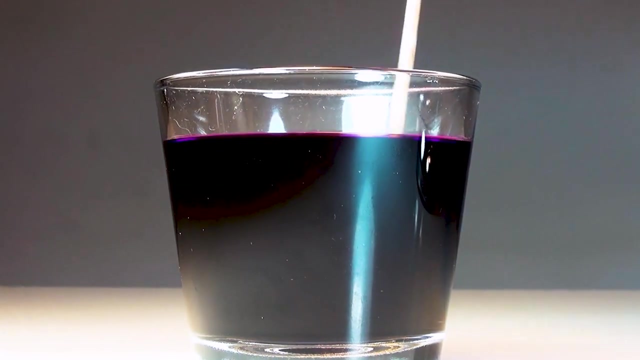 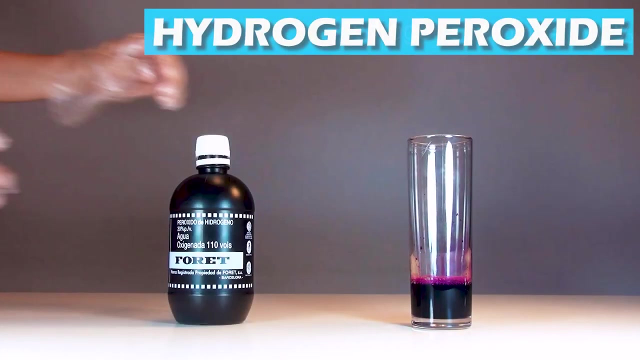 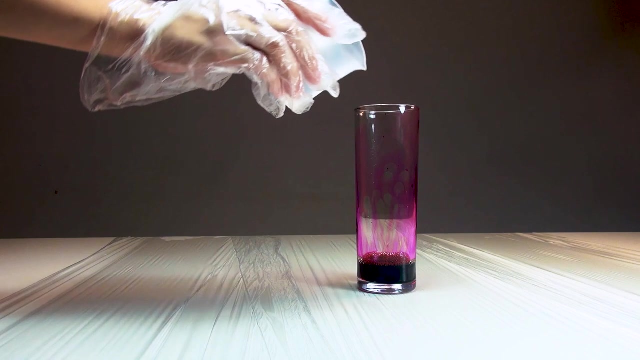 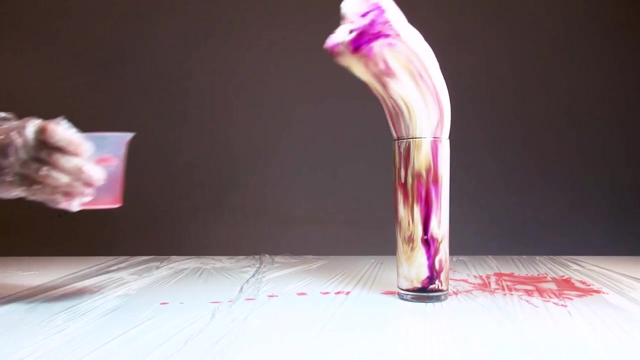 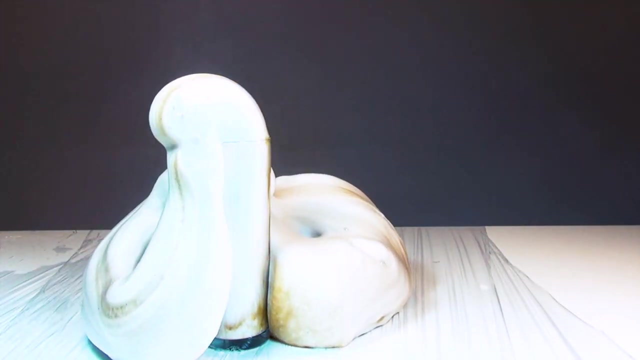 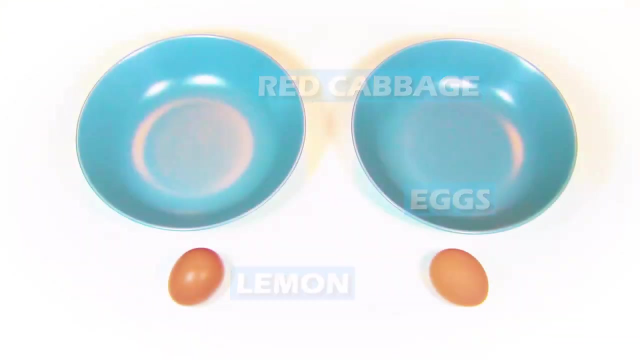 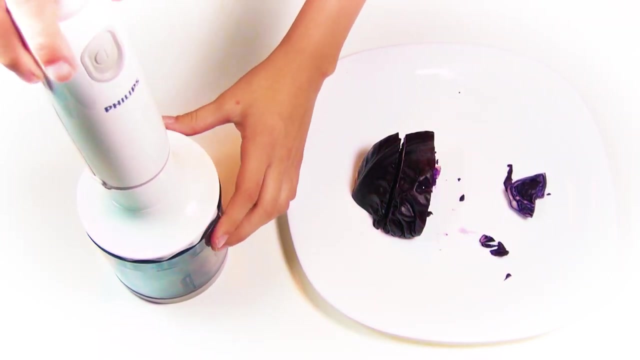 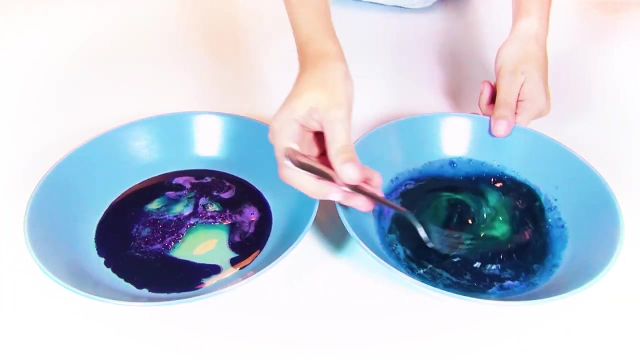 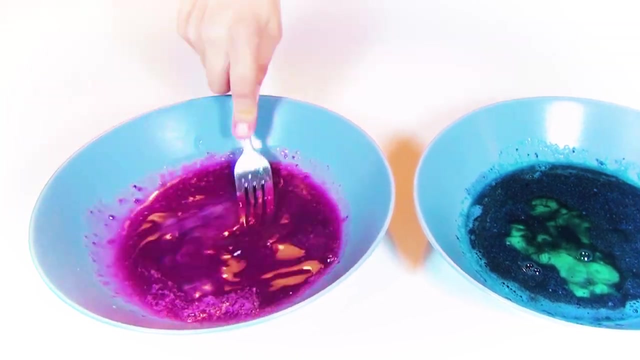 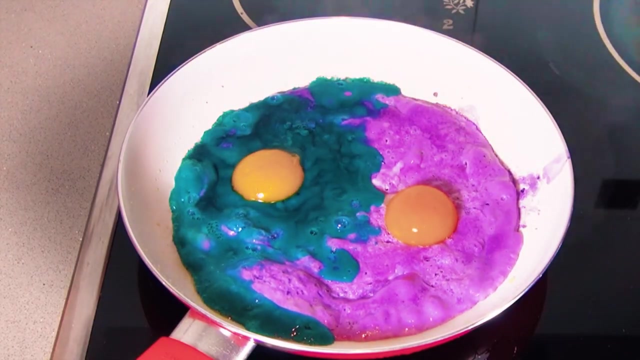 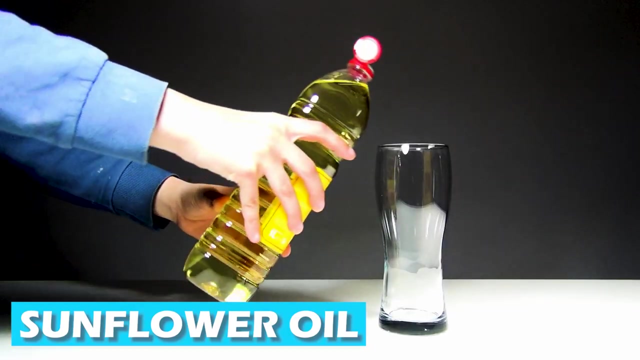 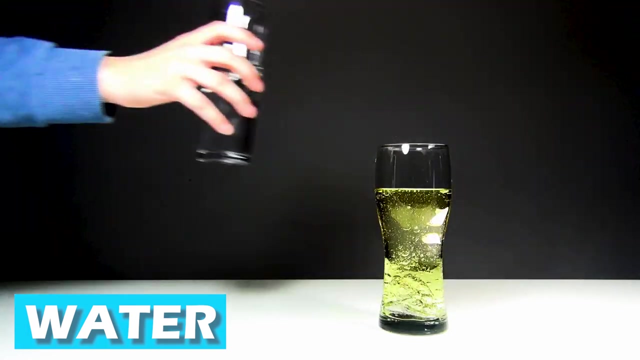 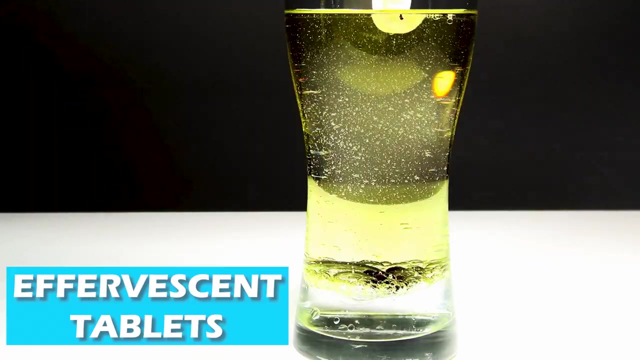 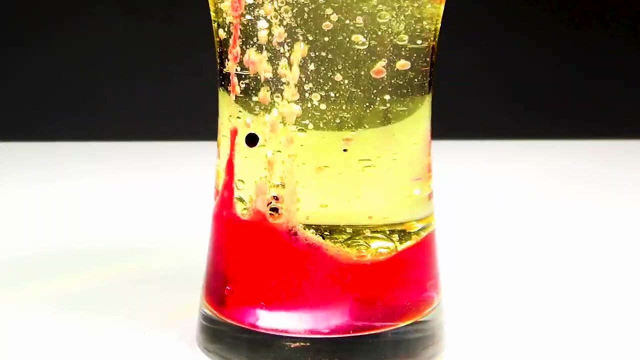 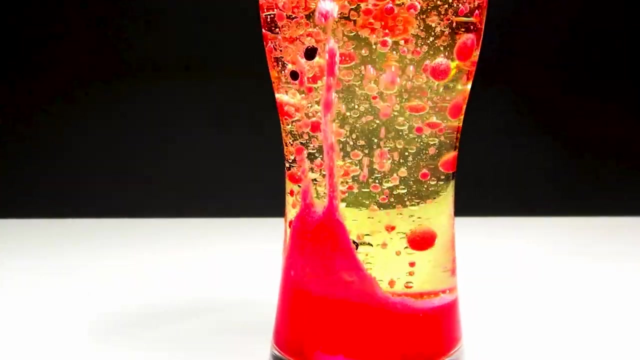 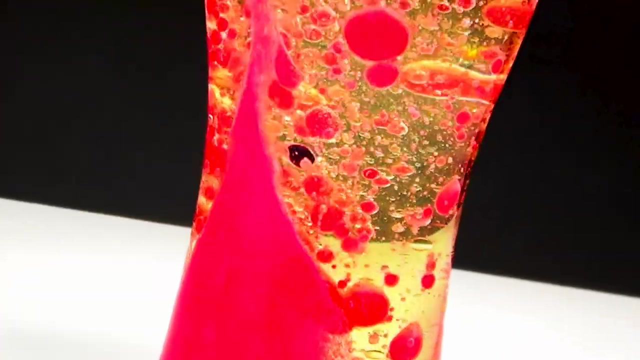 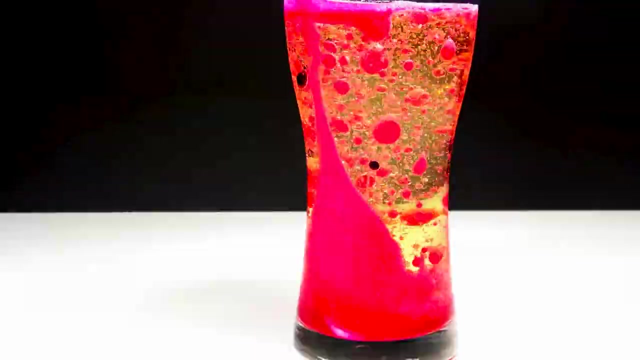 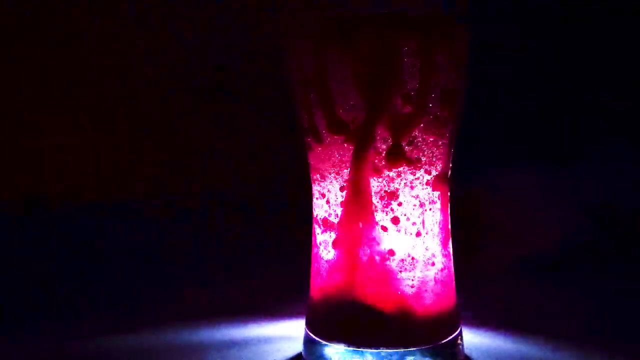 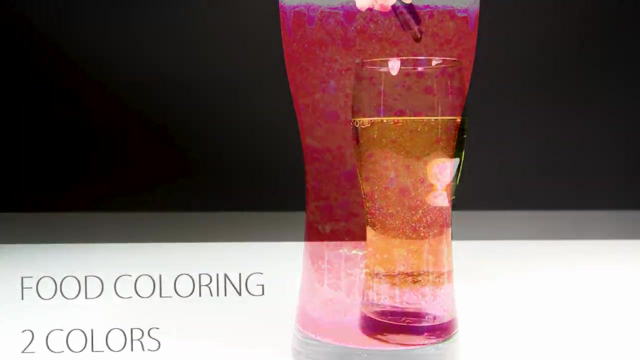 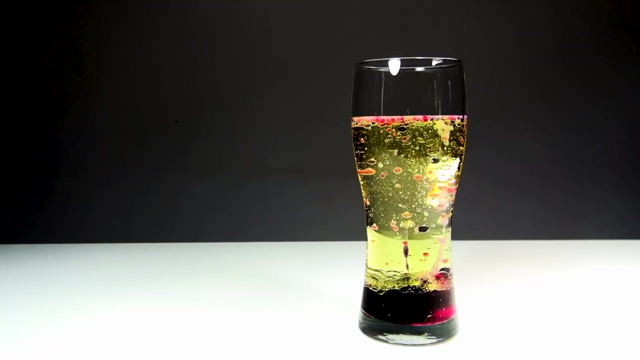 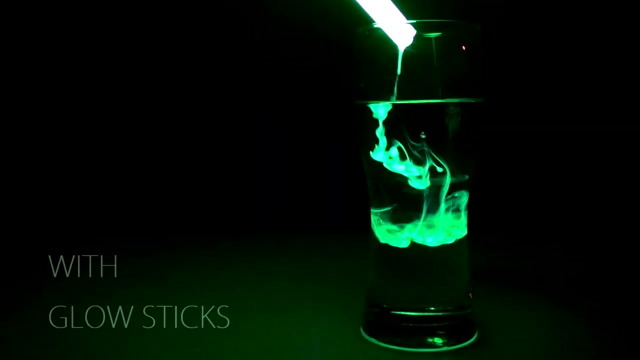 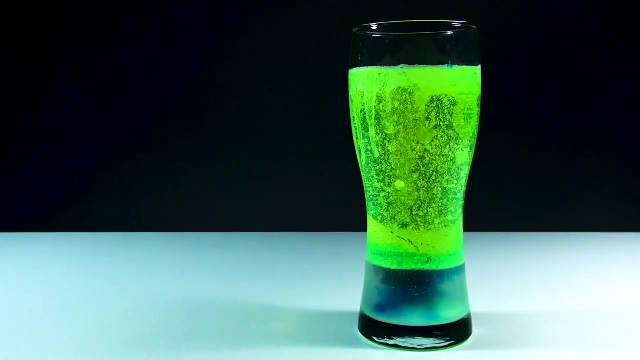 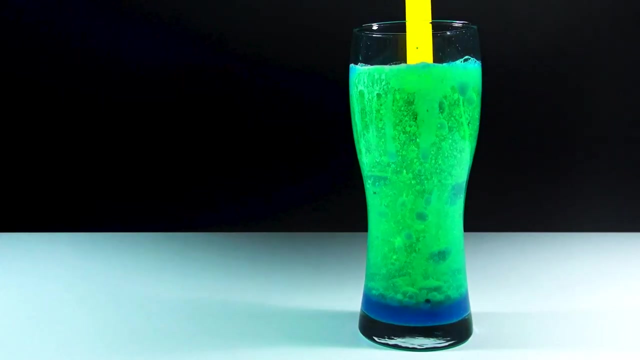 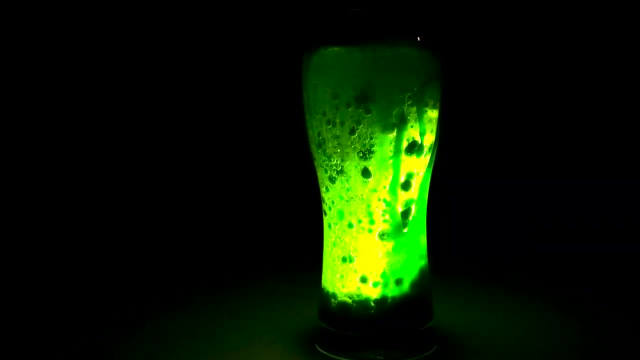 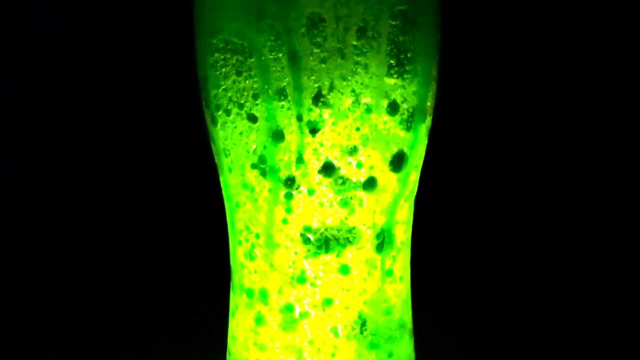 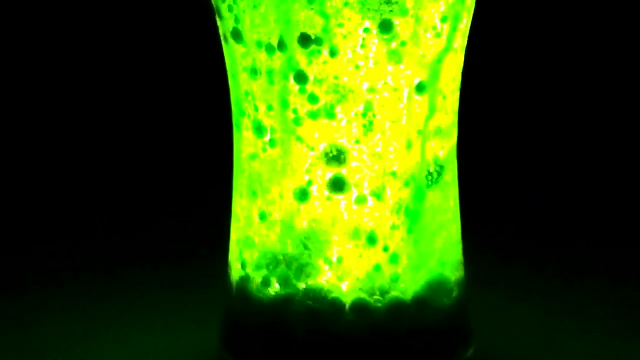